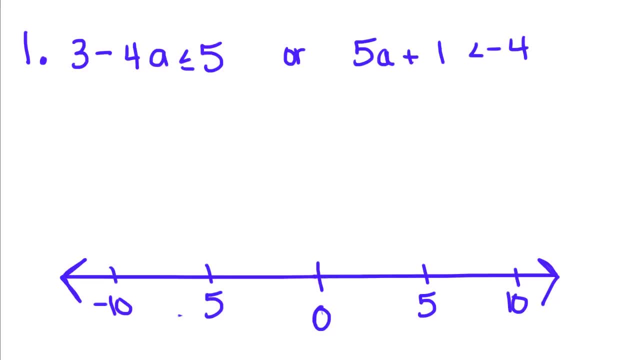 and do an example. So this is our first compound inequality, And what you need to understand is that the these two things, when they're joined by this, or make one problem. So we're going to solve each inequality separately and then, when we graph them, we're going to graph them together. 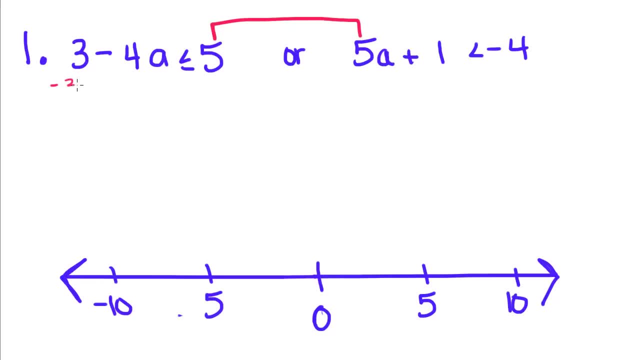 So for this we would do like we usually do: We would subtract 3 from both sides. We'd get negative 4a less than or equal to negative or to positive 2.. We divide by negative 4, we would get a greater than or equal to, because, remember, you've got to flip the sign negative. 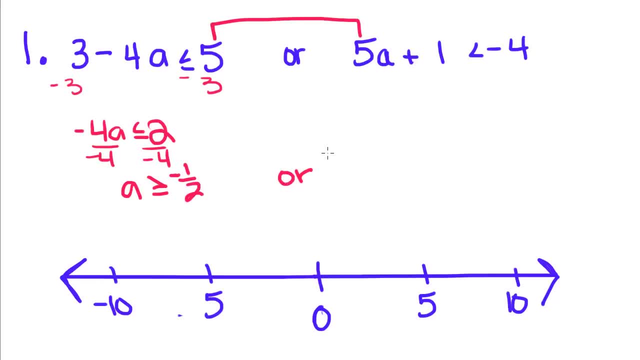 1 half, And then we're going to write or in between And we're going to solve this inequality. So 5a is less than if we subtract 1 over negative 5.. Divide by 5,, divide by 5, a is 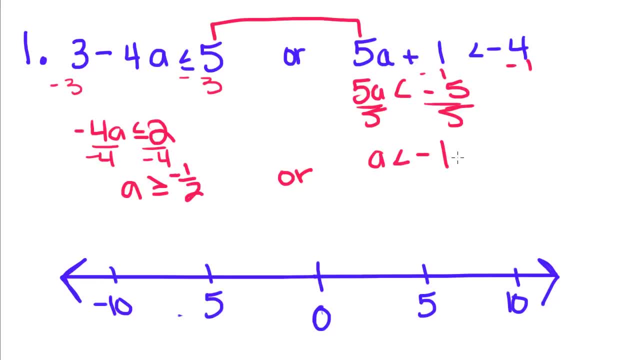 less than negative 1.. Now if, when you solve this, you get a is greater than negative 1, then you didn't realize that you only divided by positive 5.. You didn't divide by negative 5.. Just because you get a negative answer doesn't mean that you have to switch your. 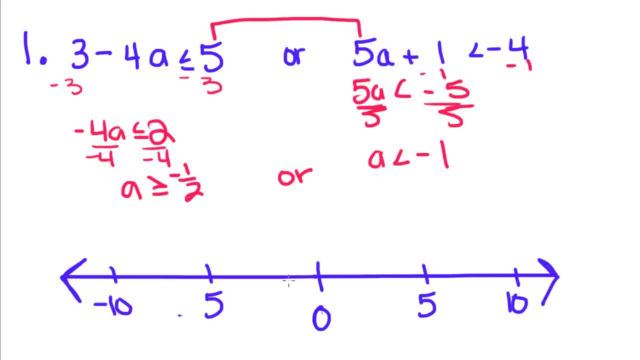 sign. So when we graph this first, we're going to plot our points for each one of these. So this is a greater than or equal to negative 1 half, Which I'm just going to have to estimate and say that negative 1 half is right here. 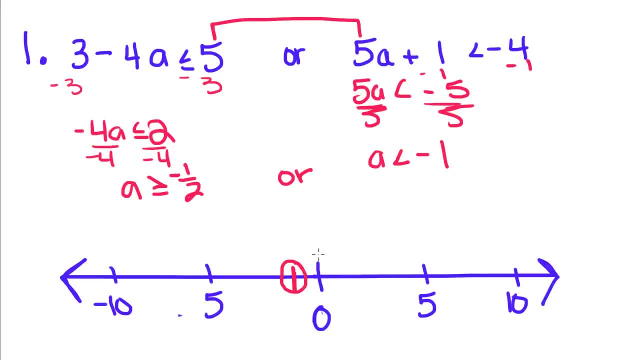 So I'm going to put a circle around that And then a less than or equal to negative 1.. Which is going to be close to 1 half. We'll say like, right there. So since I have a greater than or equal to, I'm going to have a closed circle over negative 1 half And an open circle. 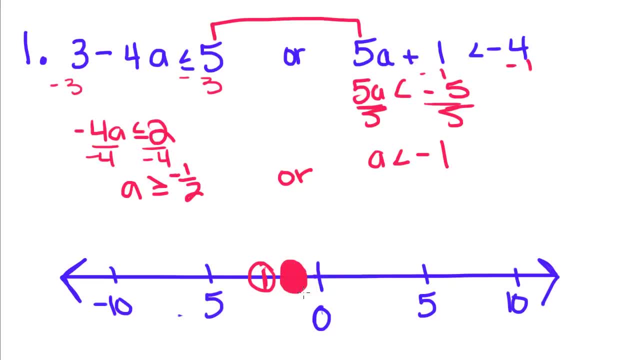 over negative 1 half And an open circle over negative 1 half And an open circle over negative 1.. Now if you look, you have to put your make sure you match your inequality up with the right point. So you have a less than negative 1 and a greater than or equal to 1 half. So 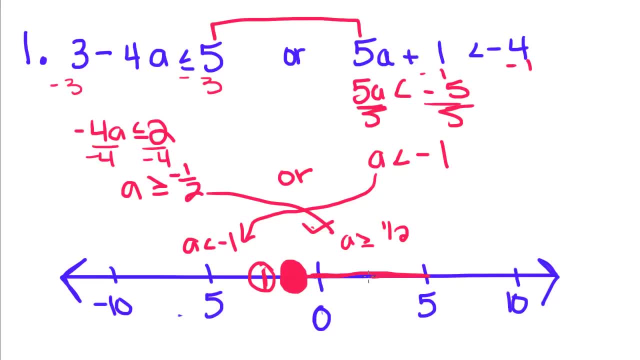 that means that this: you're going to have an arrow going this way for all your a's that are greater than 1, negative 1 half, Greater than or equal to negative 1 half, And then you're going to have an arrow pointing to the left for all a's that are less than negative. 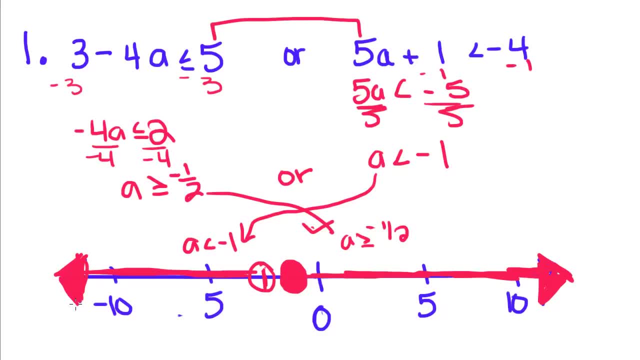 1. So when you plug in your numbers for each one of these, you're going to plug them in separately to check. So we're going to do one more example, but this time we're going to use an and compound inequality. 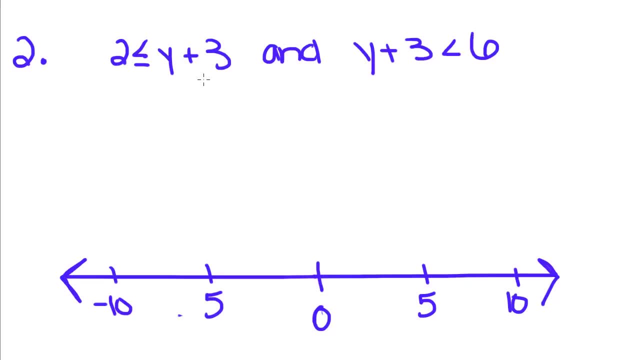 So again, we're going to solve both inequalities like we normally would. So we're going to subtract 3 from both sides, get negative, 1 less than or equal to y. So I always like to write my inequalities with the variable on the left, because that's how we graph them. 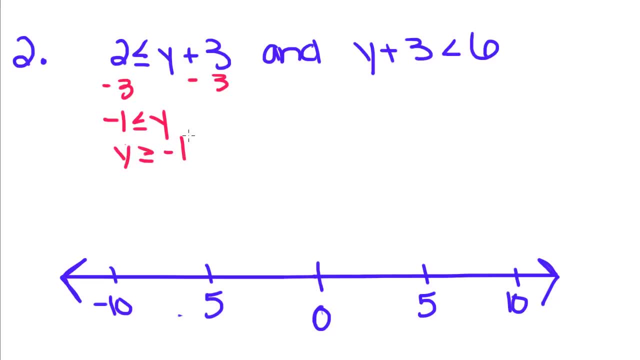 So this is y greater than or equal to negative 1.. Now, if you look, I didn't change anything about this inequality, because this inequality says that negative 1 is less than or equal to y, And this inequality says that negative 1 is less than or equal to y too. So I'm going. 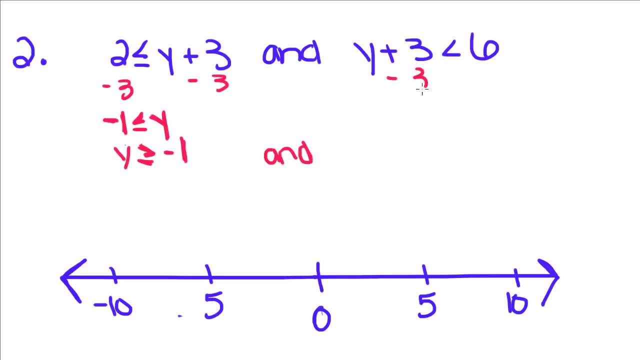 to write my and down and I'm going to solve this inequality separately. So we subtract 3 from both sides and we get y less than 2.. So first thing we're going to do is plot our points. So 2 is about right there, Negative 1 is about right there, And this one's greater than or. 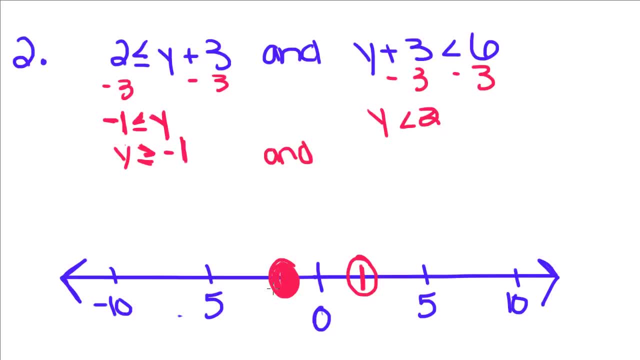 equal to negative 1.. So we're going to have a closed circle. Now this and right here is going to join these two inequalities together And we're going to shade the area in between these two circles. And because i'm a little disappointed using